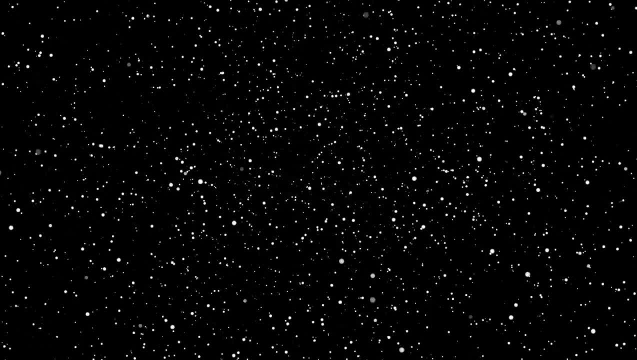 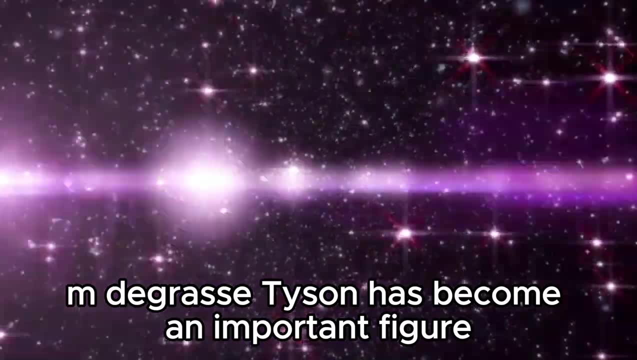 new technology brings us new ideas and perspectives. These ideas challenge what we once thought were unquestionable truths. M deGrasse Tyson has become an important figure in this changing world of science. Now something exciting is happening with the James Webb Space Telescope. 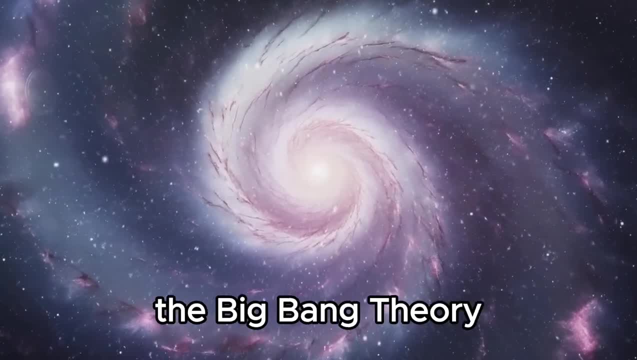 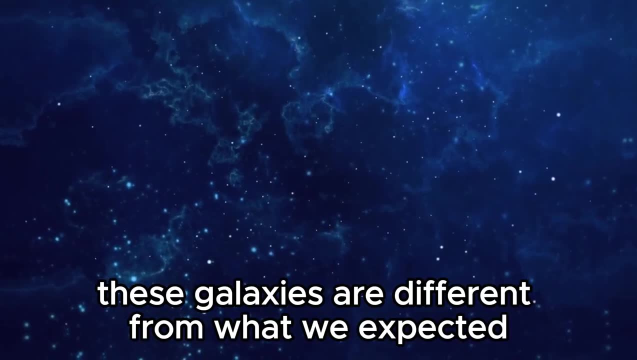 It's revealing something that might make us question the Big Bang Theory. The James Webb Space Telescope has found 750 new galaxies. These galaxies are different from what we expected, leading us to rethink what we thought we knew about them. This telescope was designed to. 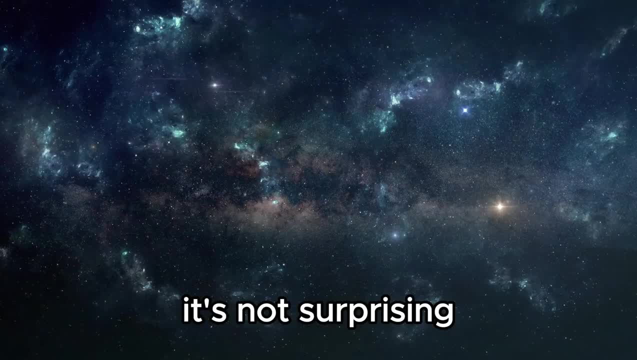 help us understand the universe. It's a great way to understand the universe. It's a great way to understand how galaxies came to be, so it's not surprising that it's shaking up our understanding of the universe. In the past, scientists said that the Big Bang Theory was the 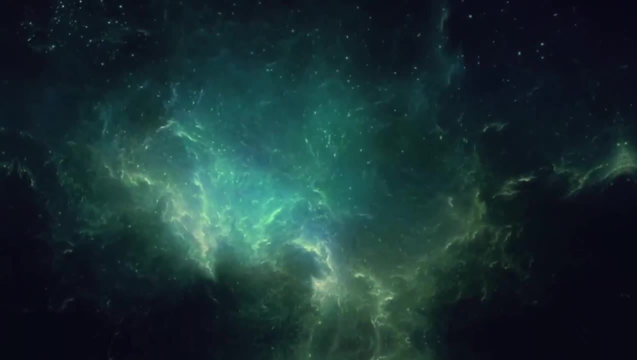 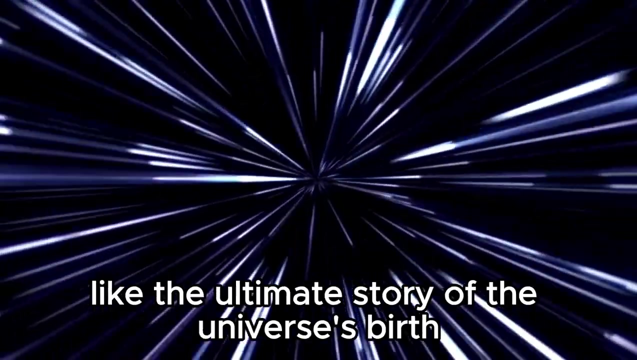 best explanation for how the universe started. According to this theory, about 14 billion years ago the universe came into being through a mysterious cosmic event, like the ultimate story of the universe's birth. But the images from the James Webb Space Telescope have challenged this. 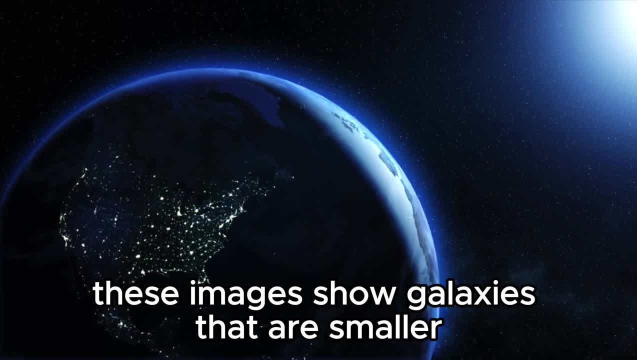 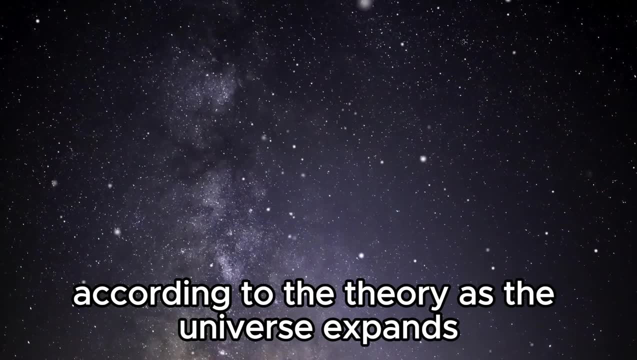 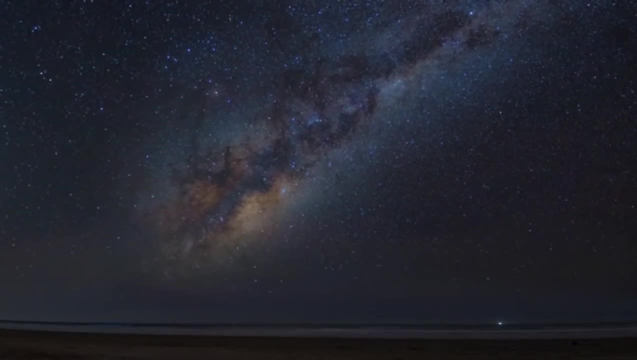 idea. These images show galaxies that are smaller, smoother, older and more numerous than what the Big Bang Theory predicts. According to the theory, as the universe expands, objects should look bigger the farther away they are, But these galaxies don't follow that rule. The theory also says that at the very beginning. 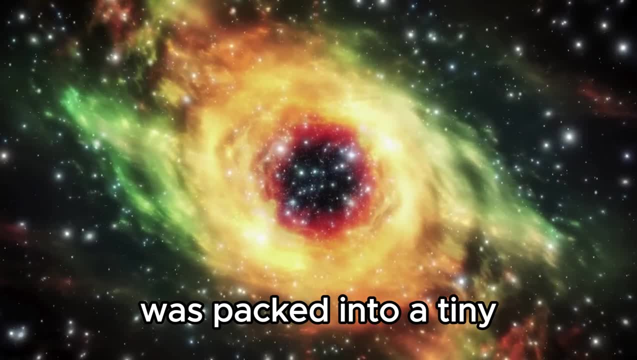 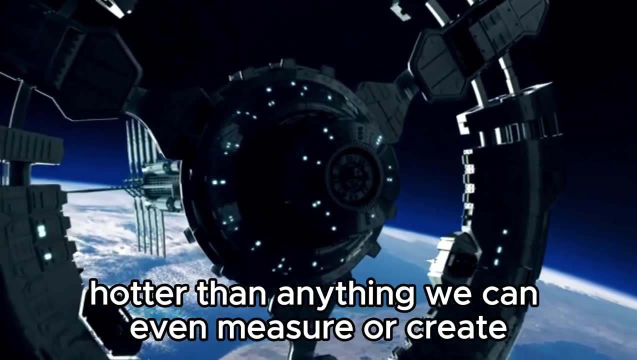 of the universe, all the stuff that makes up the cosmos, was packed into a tiny, super-dense point called a singularity. This singularity was incredibly hot, hotter than anything we can even measure or create. This idea of a singularity is a very important part of the universe. 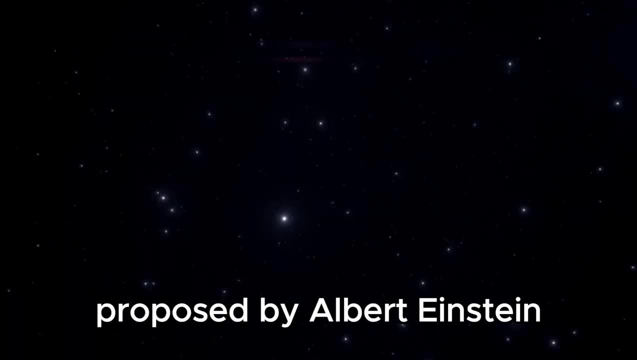 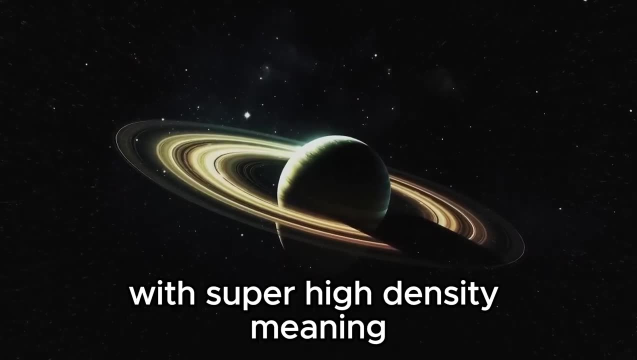 The singularity comes from a set of equations in physics proposed by Albert Einstein called general relativity. Inside the singularity, all the stuff in the universe was squeezed into a tiny space with super-high density, meaning there was an enormous amount of mass and energy packed. 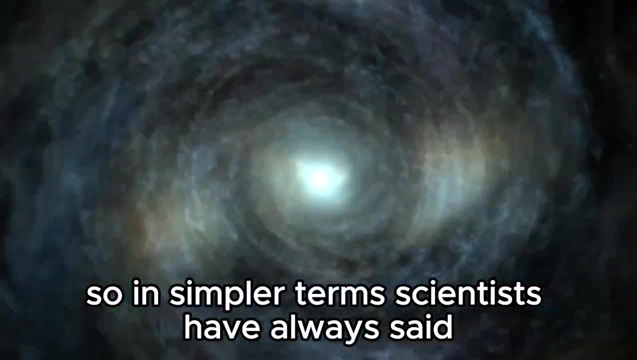 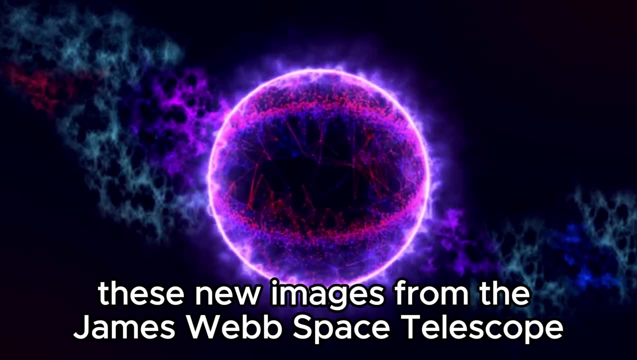 into a tiny space. So, in simpler terms, scientists have always said the Big Bang Theory was how the universe started, But now these new images from the James Webb Space Telescope are making us question that idea. The galaxies it found in the universe are the ones that make up the universe. 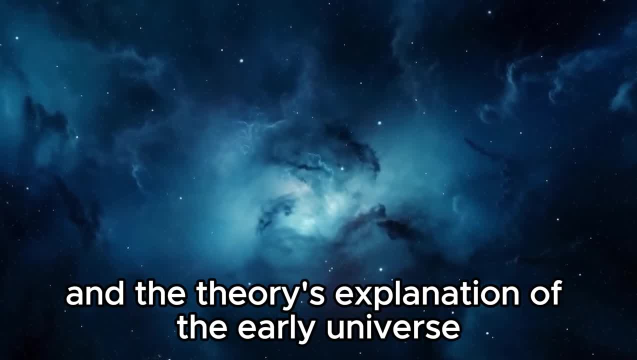 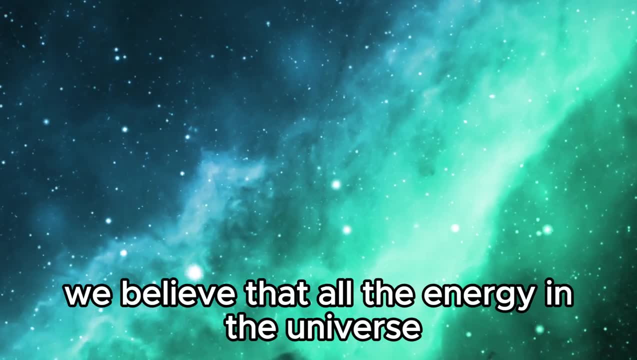 That's why you can enjoy the theory a lot. Let's begin together in the first minute. looking at our own life, You can imagine that the universe could have existed more before 100,000 years ago if we could see it today. when we do this, While we may wonder what the 골�ney-mconfidence? 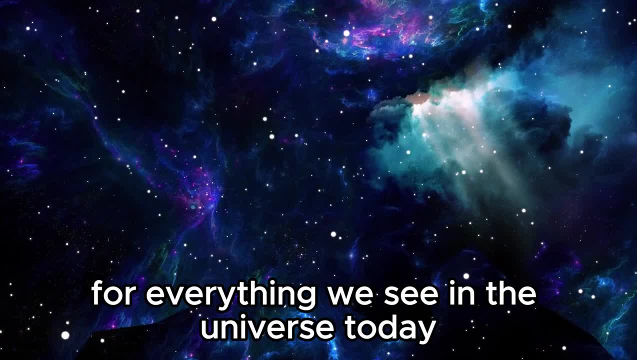 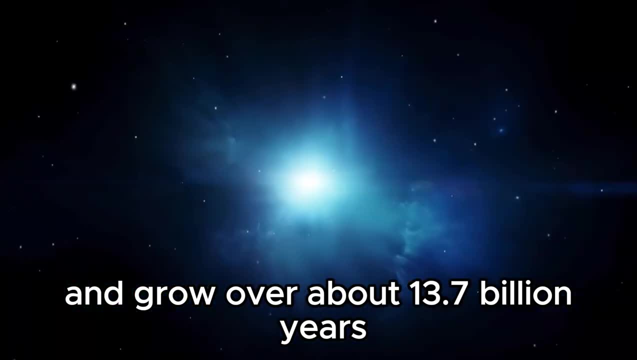 of Mars was. it cannot be determined with a single gesture. At first, we believe it existed only out of spent time, And even the human world itself has a history relatively differentアögε chordه, Or three million years ago. Let's guess that there were five years ago when Mars existed- not just today, butready. 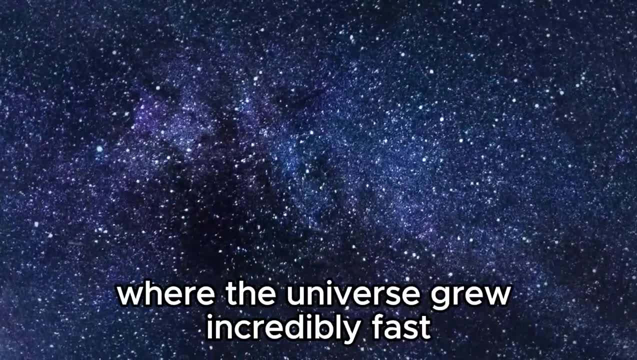 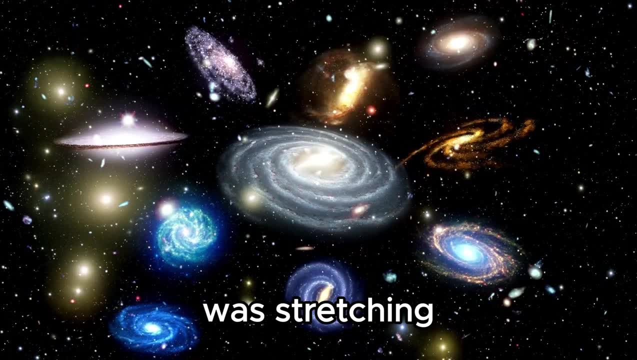 and started with something called cosmic inflation, where the universe grew incredibly fast, even faster than the speed of light. It's like the very fabric of space itself was stretching and everything in it was stretching along with it. This cosmic inflation helped shape the universe. 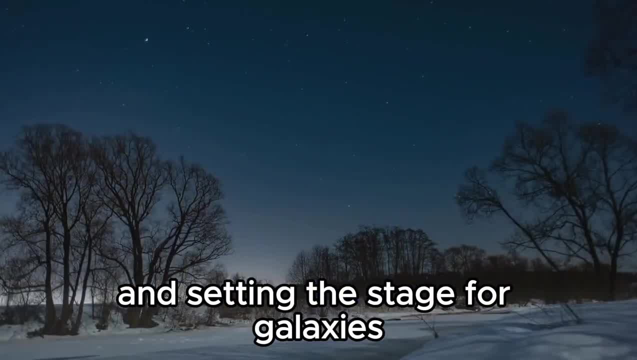 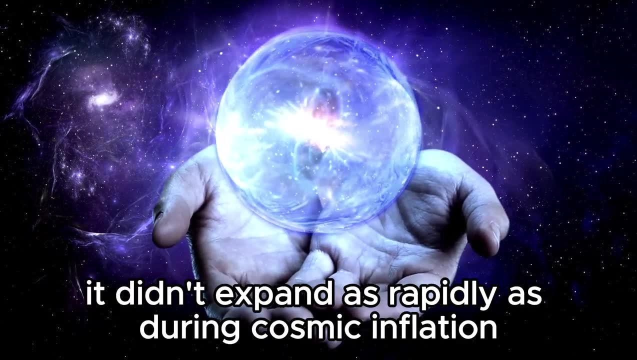 by making things more uniform and setting the stage for galaxies, stars and other cosmic structures to form As the universe continued to expand. it didn't expand as rapidly as during cosmic inflation, but it still kept getting bigger. We call this ongoing expansion cosmic. 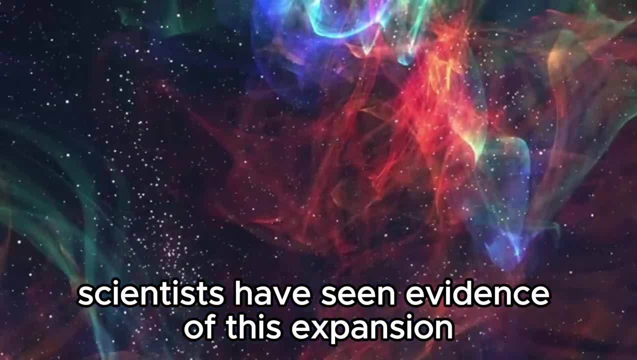 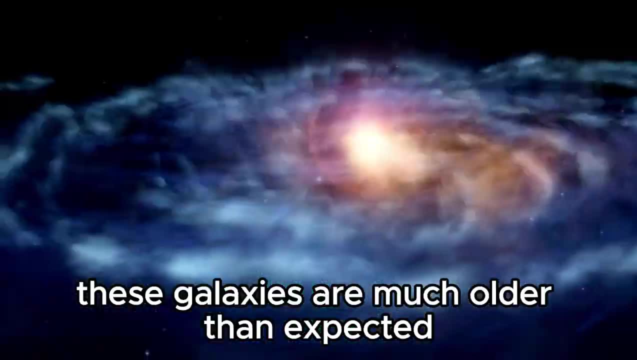 expansion. Scientists have seen evidence of this expansion through things like the way light from distant galaxies changes color, known as redshift. First of all, these galaxies are much older than expected. This challenges what we thought we knew about how galaxies form and evolve according to 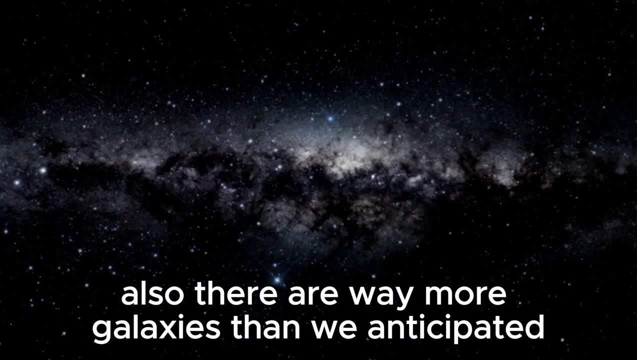 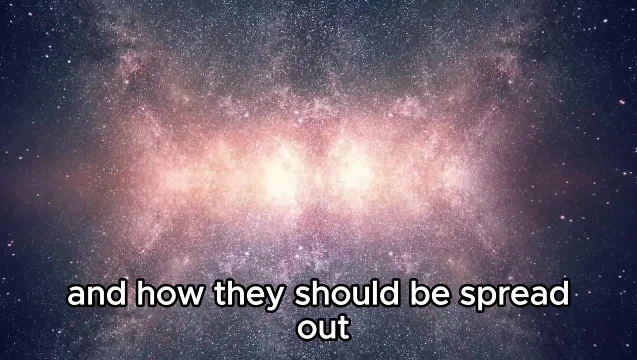 the Big Bang Theory. Also, there are way more galaxies than we anticipated. The Big Bang Theory is a theory of the universe. It's a theory of the universe. It's a theory of the universe. The Big Bang Theory made predictions about how many galaxies there should be and how they should. 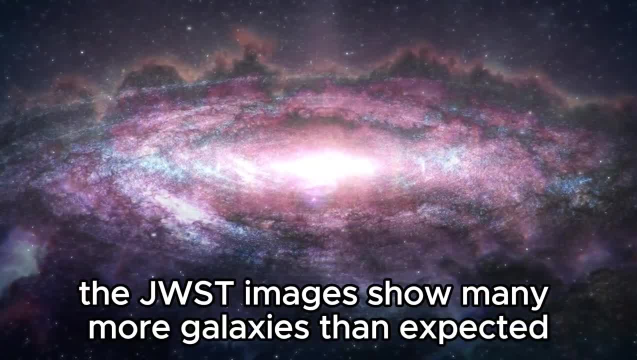 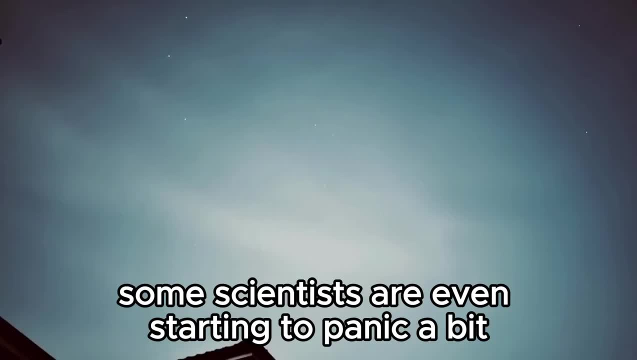 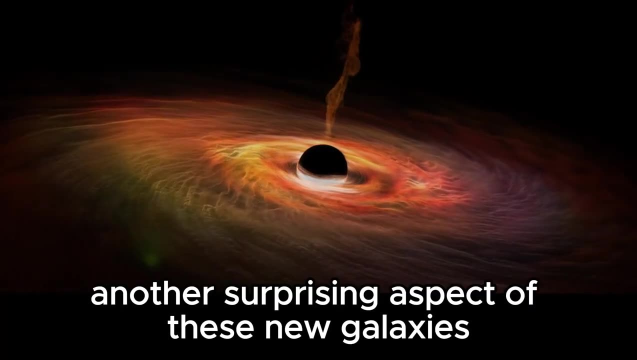 be spread out, but the JWST images show many more galaxies than expected. This makes scientists question whether the theory's predictions are accurate. Some scientists are even starting to panic a bit because these findings don't match their expectations at all. Another surprising aspect of these new galaxies is their smoothness, which goes against what the Big Bang Theory 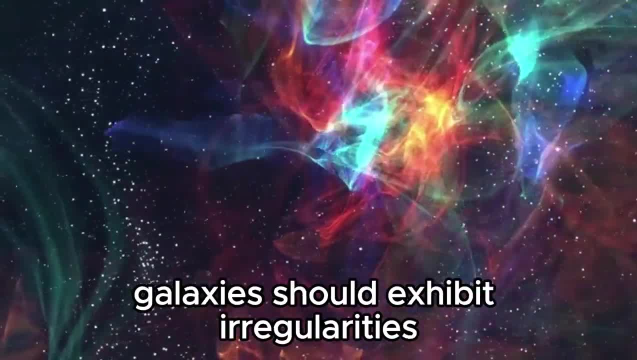 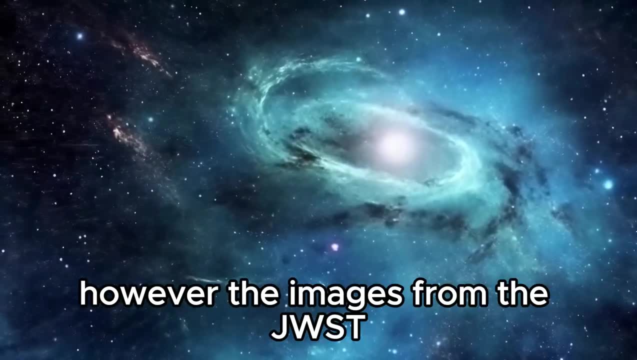 suggests. According to the theory, galaxies should exhibit irregularities. The Big Bang Theory suggests that galaxies have irregularities and variations in their structures due to how they formed and evolved. However, the images from the JWST show galaxies that are unusually smooth. 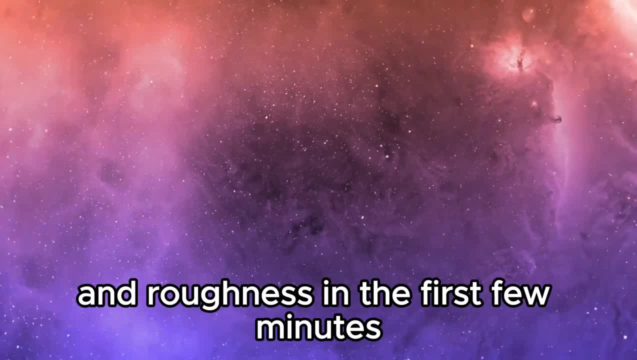 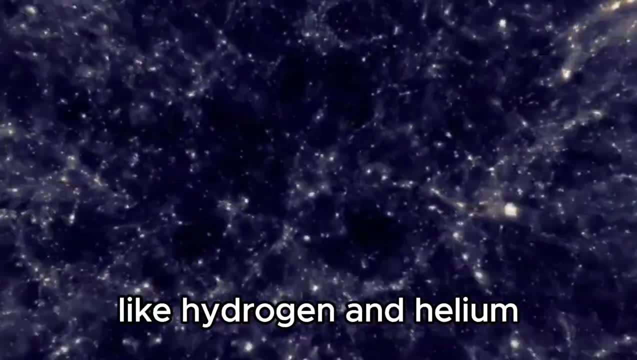 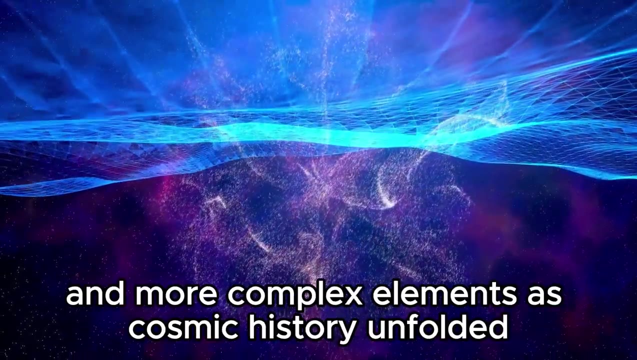 lacking the expected complexity and roughness. In the first few minutes after the Big Bang, there was a process called nucleosynthesis, which involved the creation of lightweight elements like hydrogen and helium. These elements set the stage for the formation of stars, galaxies and more complex elements As cosmic history unfolded. 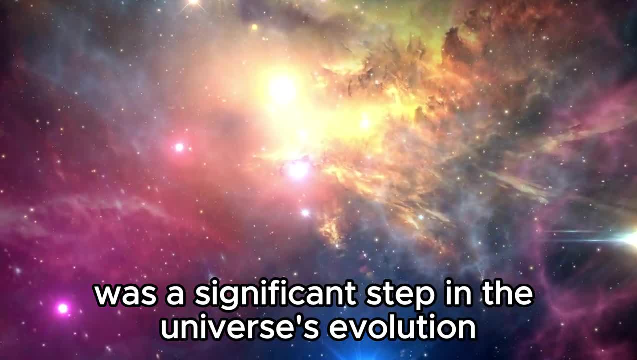 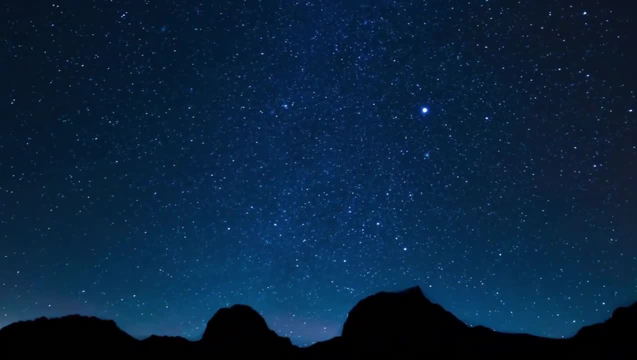 the synthesis of elemental building blocks was a significant step in the universe's evolution, transitioning from a primordial sea of particles and energy to a state where matter began to take shape. The Big Bang Theory had anticipated seeing galaxies that were jumbled and disrupted due to 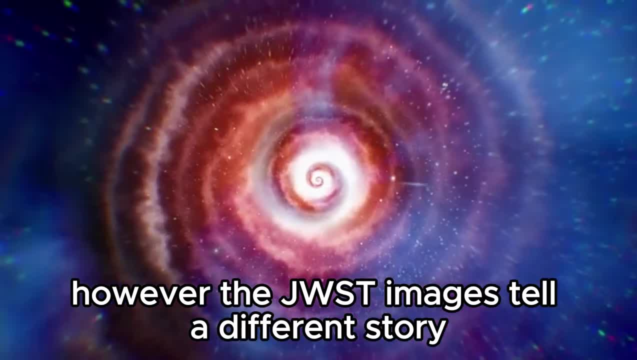 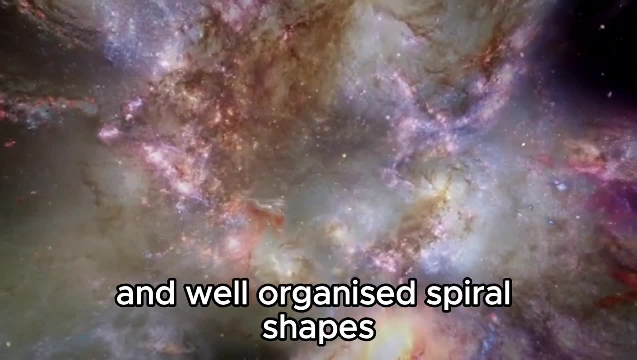 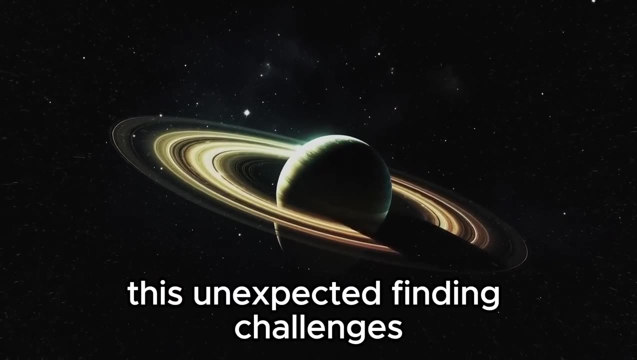 multiple collisions. However, the JWST images tell a different story. Instead of chaotic and disordered galaxies, the pictures reveal smooth disks and well-organized spiral shapes resembling the galaxies observed in the present-day universe. This unexpected finding challenges the idea that mergers are a common part of galaxy evolution. 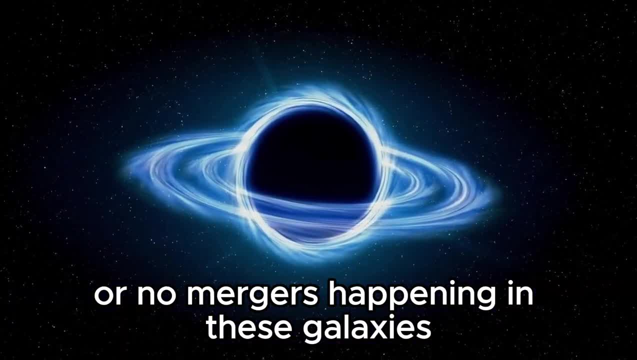 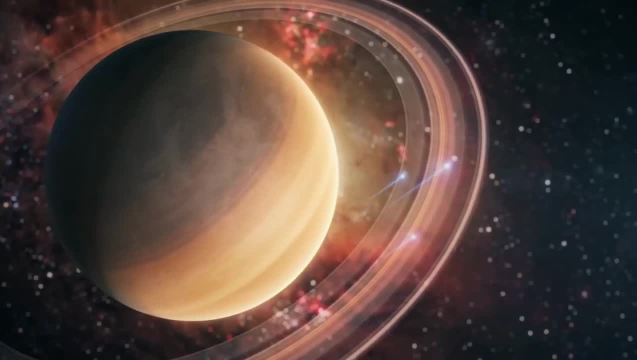 If there are very few or no mergers happening in these galaxies, as suggested by the Big Bang Theory, it becomes unlikely that tiny galaxies could grow to become hundreds of times larger. According to the theory, the universe began in a super hot and dense state and then gradually. 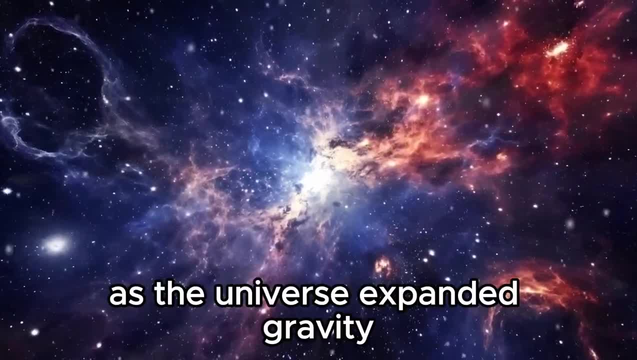 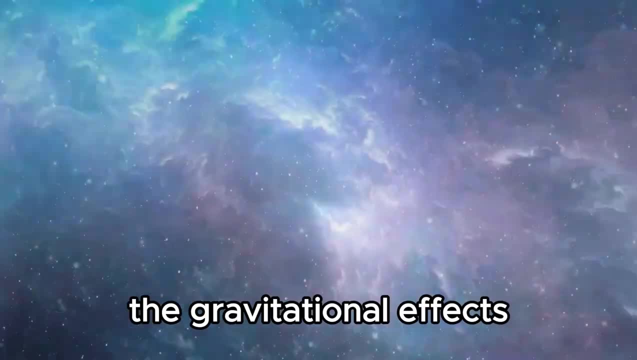 expanded and cooled down over time. As the universe expanded, gravity played a crucial role in shaping how matter was distributed and formed. The universe expanded and cooled down over time. The gravitational effects predicted by the Big Bang Theory are consistent with what we see today. 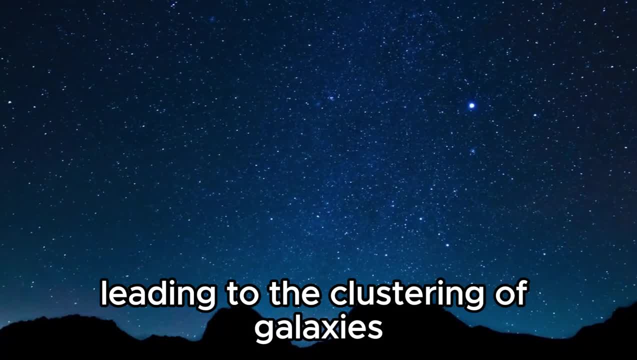 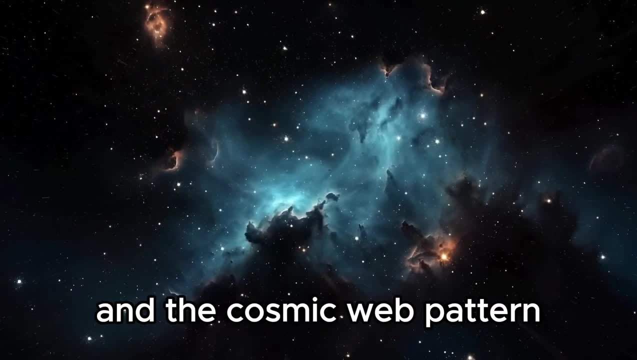 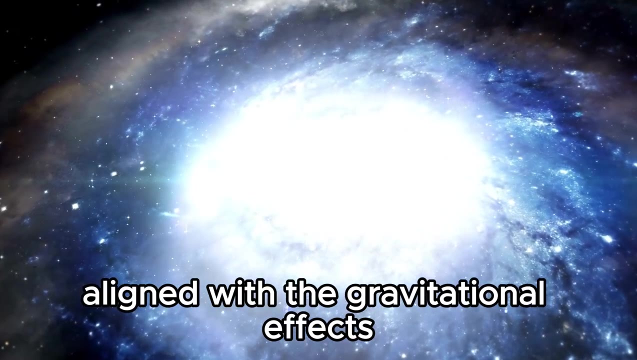 with gravity pulling matter together, leading to the clustering of galaxies and the formation of interconnected filamentary structures, known as the cosmic web. The presence of these galaxy clusters and the cosmic web pattern strongly supports the Big Bang Theory. The way galaxies are distributed across the universe aligns with the gravitational effects expected from the initial dense and 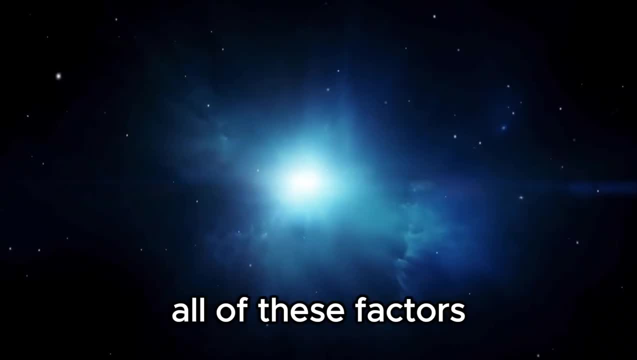 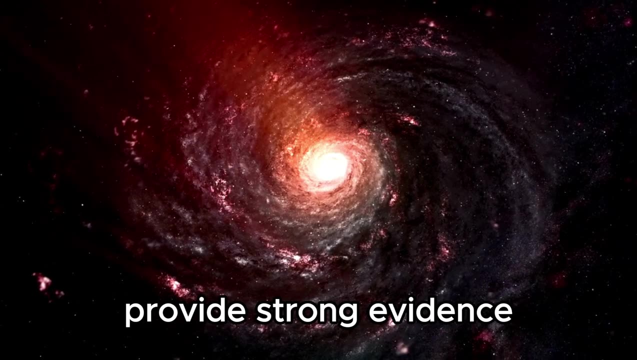 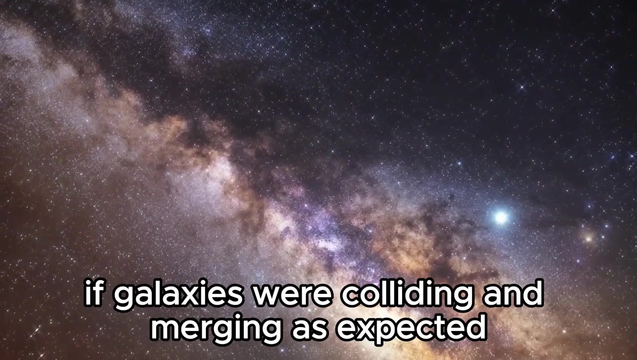 expanding state proposed by the theory. All of these factors, including the clustering of galaxies, the cosmic web structure and the distribution of galaxy clusters, provide strong evidence that the universe evolved from an extremely dense state and has been expanding over billions of years. If galaxies were colliding and 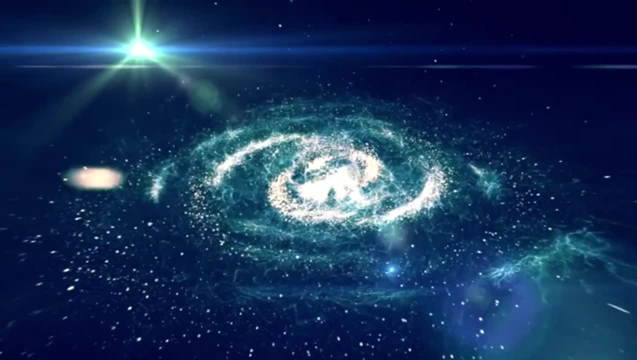 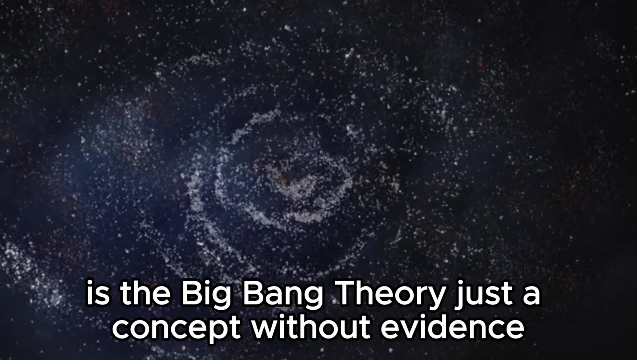 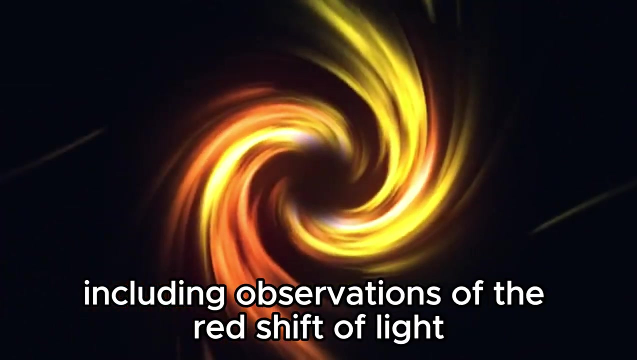 merging as expected, we would see evidence of these collisions Or dense in the interacting galaxies, But the images show something different. So is the Big Bang Theory just a concept without evidence? No, it is actually supported by compelling evidence, including observations of the redshift. 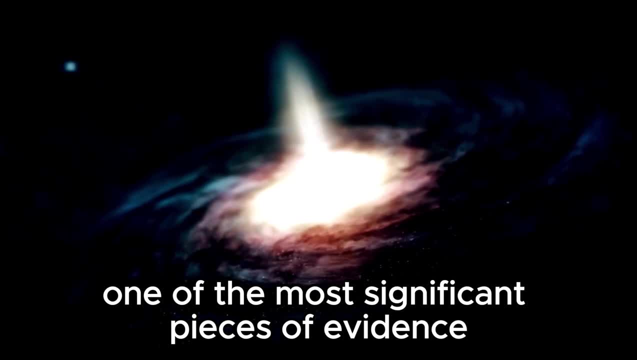 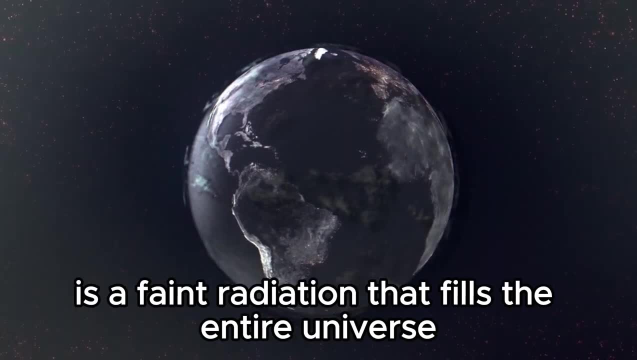 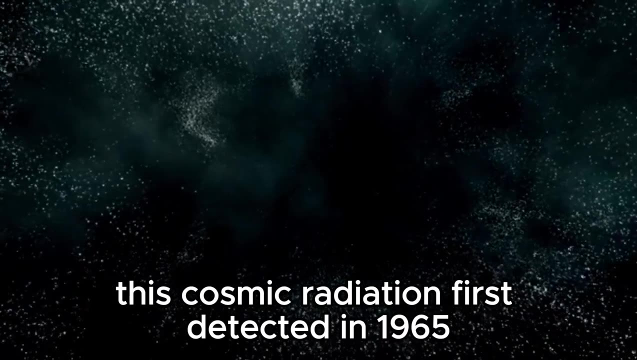 of light. One of the most significant pieces of evidence for the Big Bang Theory is the discovery of the Cosmic Microwave Background CMB. The CMB is a faint radiation that fills the entire universe and represents the afterglow of the Big Bang. This cosmic radiation first. 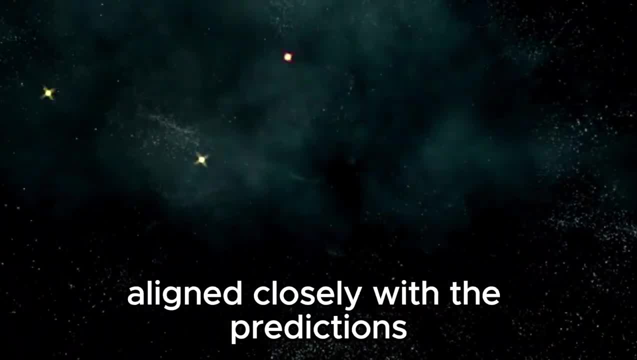 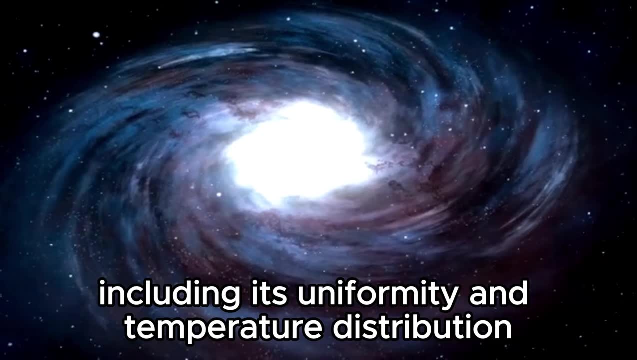 detected in 1965, aligns closely with the predictions made by the Big Bang Theory. The observed characteristics of the CMB are the following: The CMB is a faint radiation that does not reflect light. The CMB, including its uniformity and temperature distribution strongly. 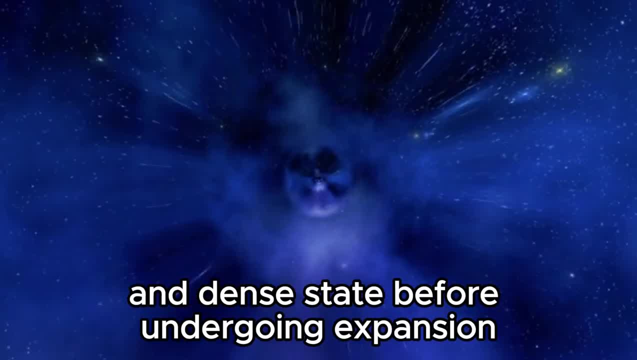 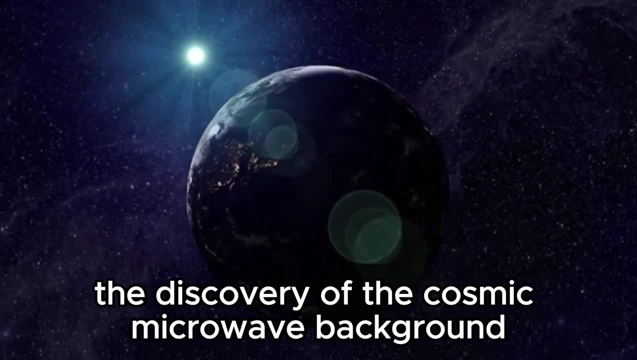 support the idea that the universe was once in an extremely hot and dense state before undergoing expansion, a central element of the Big Bang Theory. The discovery of the Cosmic Microwave Background is a crucial piece of evidence that offers us a unique glimpse into the early moments. 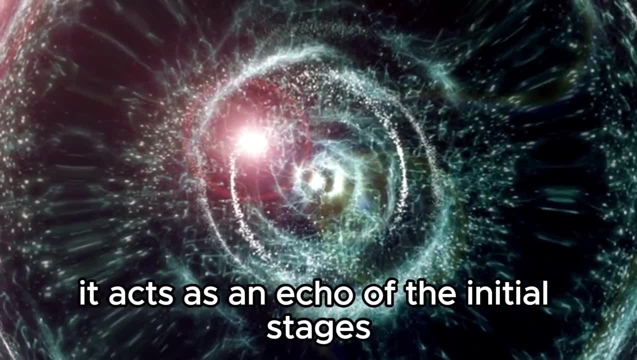 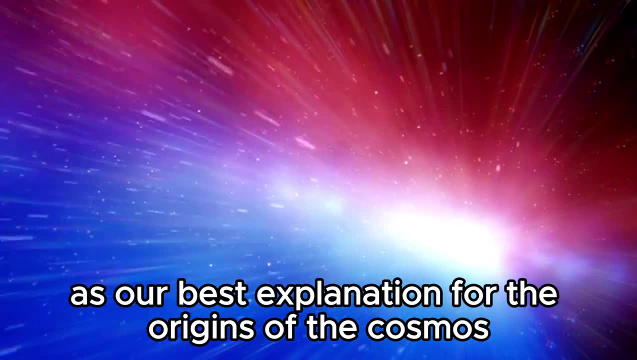 of the universe. It acts as an echo of the initial stages following the Big Bang and has played a vital role in solidifying the Big Bang Theory as our best explanation for the origins of the cosmos. However, recent findings have challenged some aspects of the Big Bang Theory: The existence of 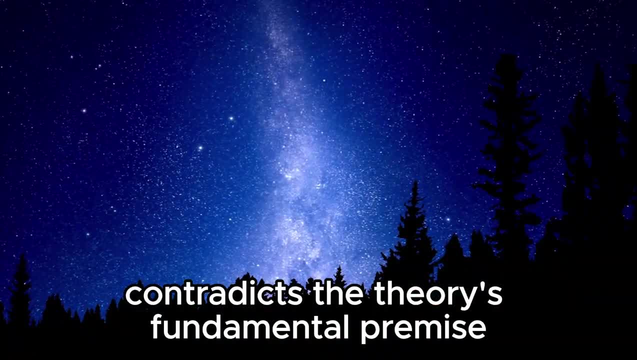 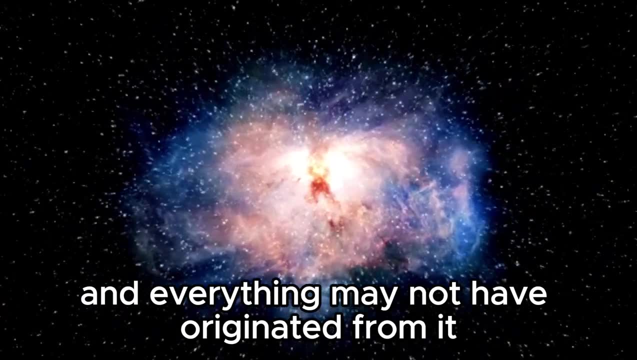 galaxies with ages that seem to predate the Big Bang contradicts the theory's fundamental premise suggesting that the Big Bang may not have occurred as originally thought and everything may not have originated from it. Proponents of the Big Bang Theory had expected that, as the James 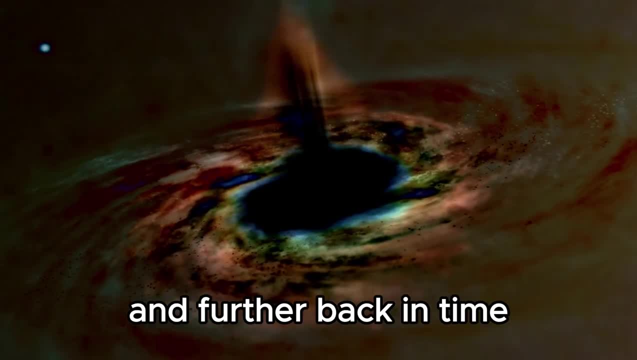 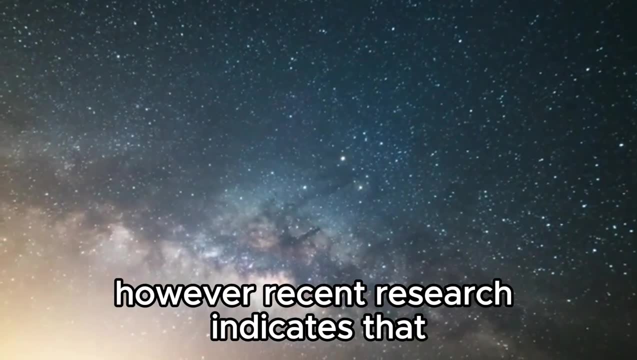 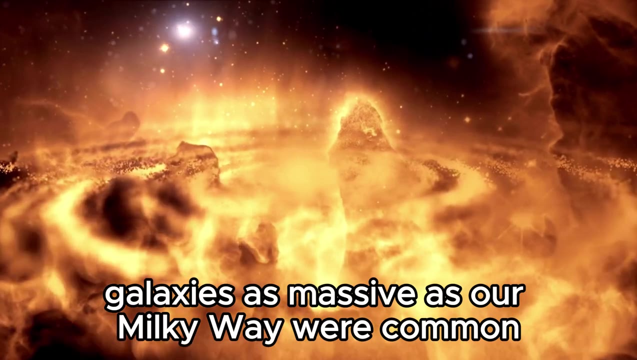 Webb Space Telescope looked further into space and further back in time, the number of observable galaxies would decrease, eventually leading to a cosmic dark age. However, recent research indicates that even a few hundred million years after the hypothetical Big Bang, galaxies as massive as our Milky Way were common. The JWST images reveal a much greater 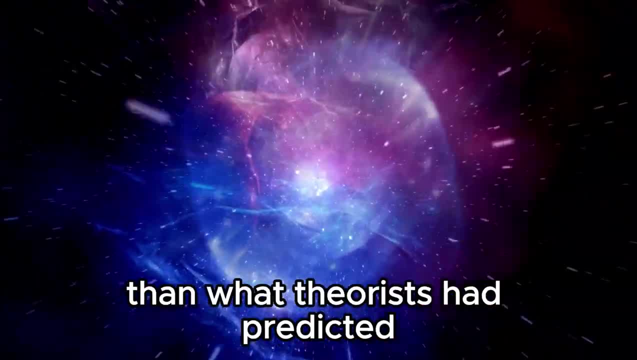 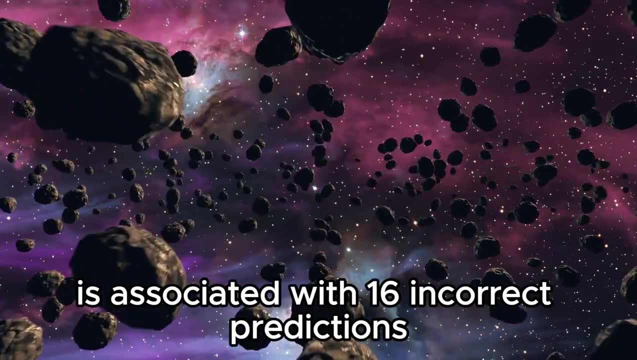 abundance of large galaxies at redshifts greater than 10 than what theorists had predicted, challenging the plausibility of the Big Bang Theory. Moreover, the Big Bang Theory is associated with 16 incorrect predictions in the current body of scientific literature, with only one 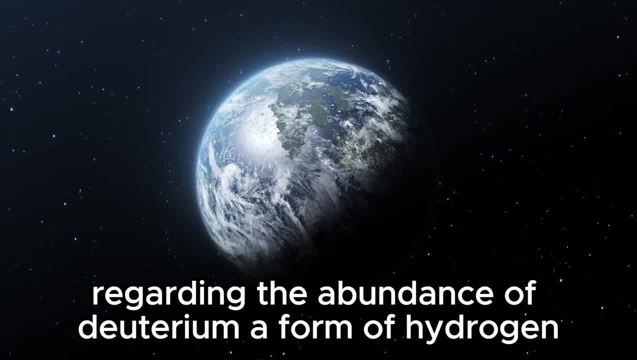 accurate prediction regarding the abundance of deuterium, a form of the Big Bang Theory. The Big Bang Theory is a form of hydrogen.